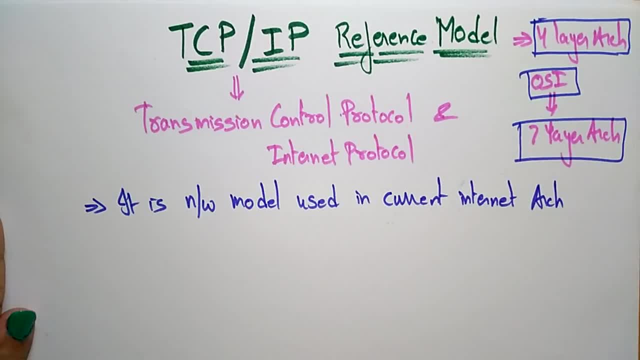 So nowadays, whatever the internet architectures we are using, So those internet or reference, this TCP, IP reference model rather than OSI reference model. okay, so actually it was developed by the Department of Defense project research agencies. let me write that point. it was developed by Department of Defense project research agency. why they are developed, this TCP? 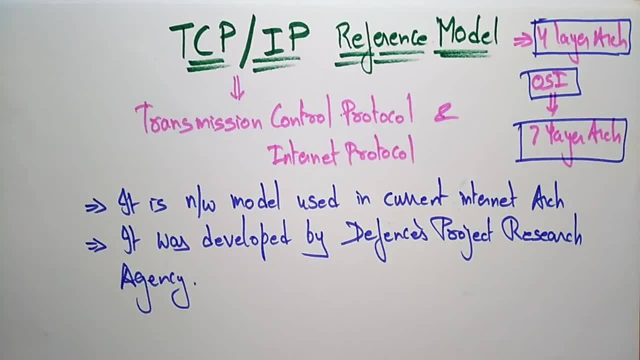 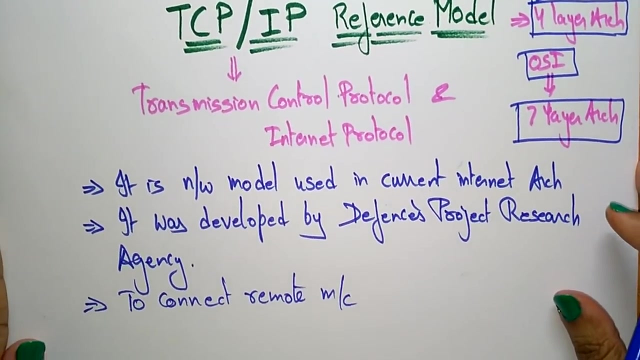 IP reference model. so as a part of research project of network interconnections- they are you, they are- developed this TCP IP to connect the remote machines. so mainly to connect remote machines, to connect remote machines. so they developed this TCP IP reference model. what is the main idea behind this TCP IP? 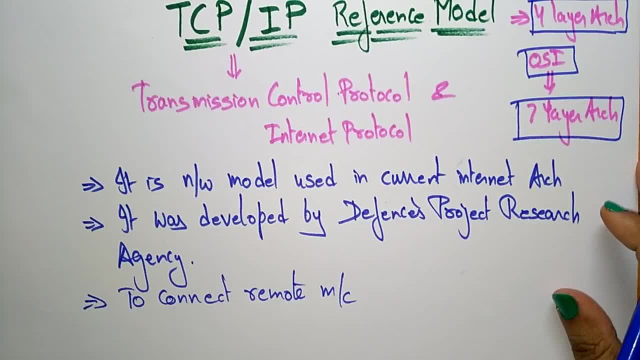 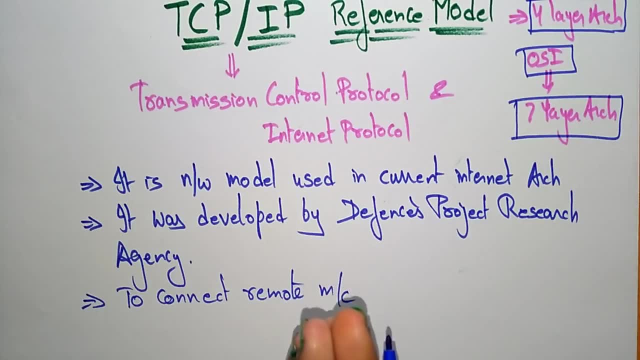 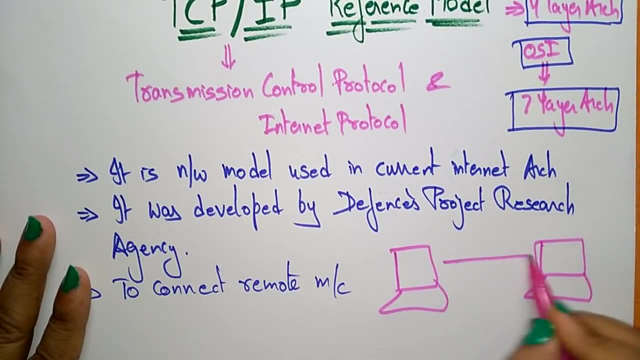 reference model. so the main idea of this TCP IP was to allow one application on one computer to send data packets or to talk to another application on running on different computer. so this is one computer somewhere and this is another computer somewhere else to transmit the data from one. 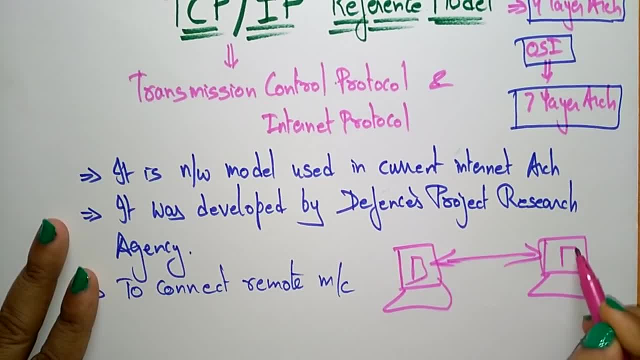 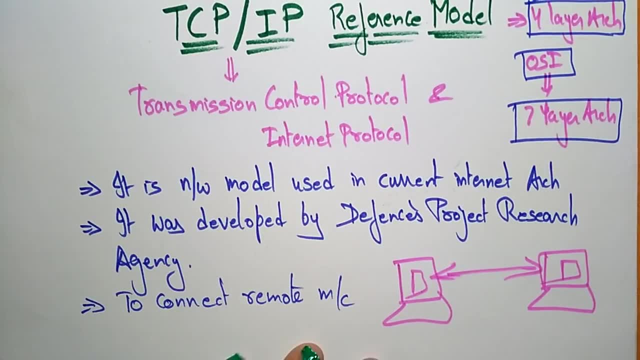 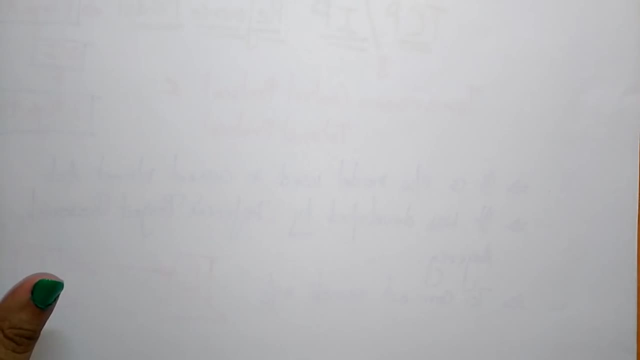 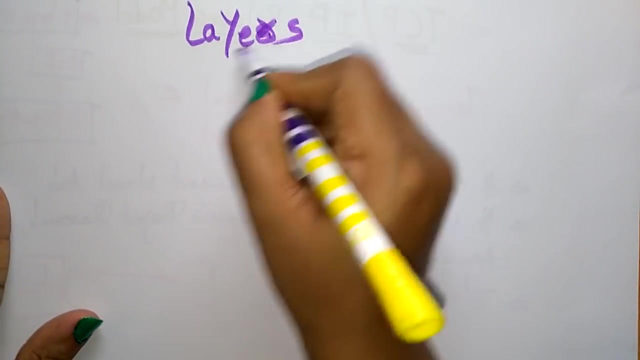 system to another system, from one system to the another system. we are using this TCP IP reference model. okay, now let us see what are the layers that are present in this TCP IP. let me write that point. the layers that are presenting layers in this TCP IP reference model are the same as other models. but 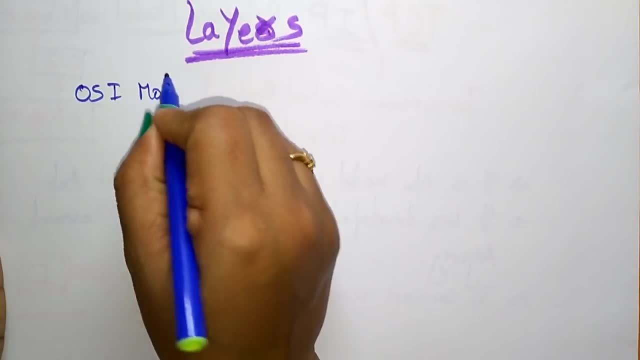 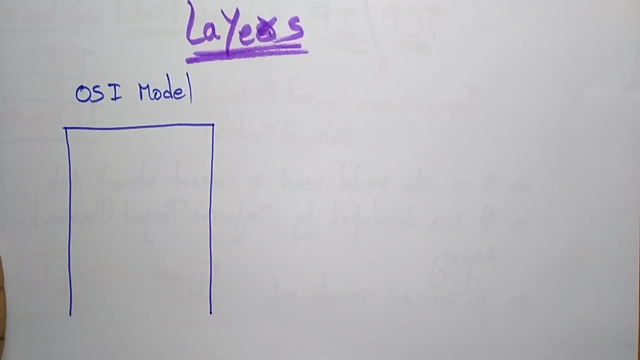 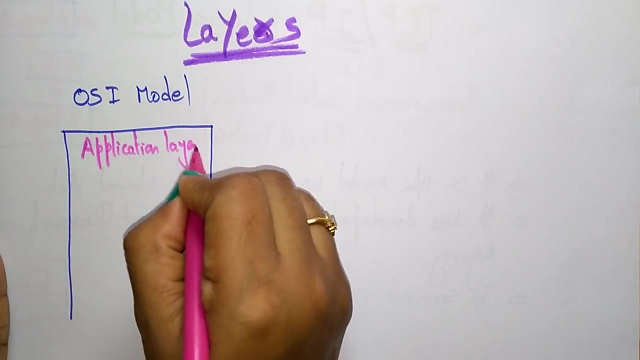 there are no further layers present. so let me write exactly exactly what is your proposal. tobility tells that the layers are present, whether from the database or so if you take the OS in request model, what other layers that will present in OS? I reference model totally. it is having the seven layers. money's. 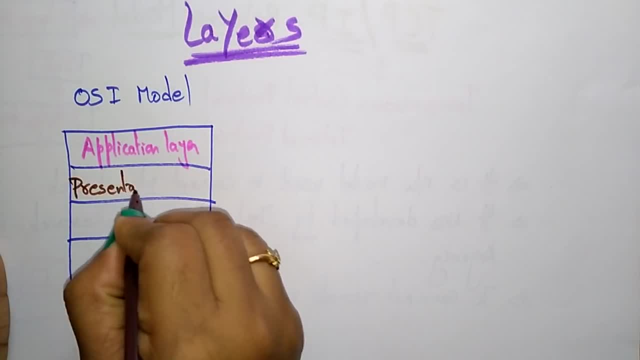 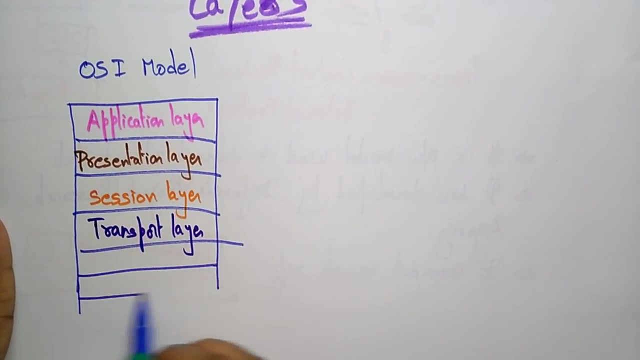 application, lay them okay. and next user presentation layer, next session layer and next transport layer, next network layer, data link layer and the final one is the physical layer. so these are the steps. total seven layers that are present in OSI reference model. so this we already discussed. now next, coming to the next. 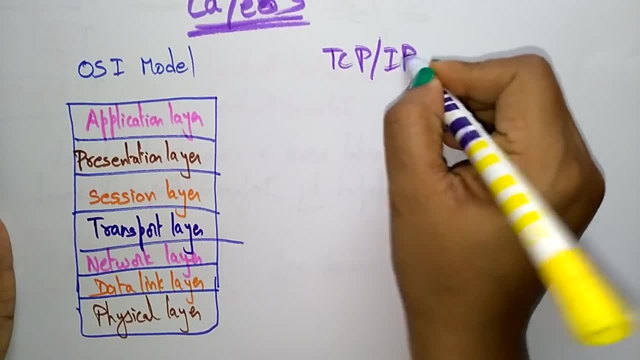 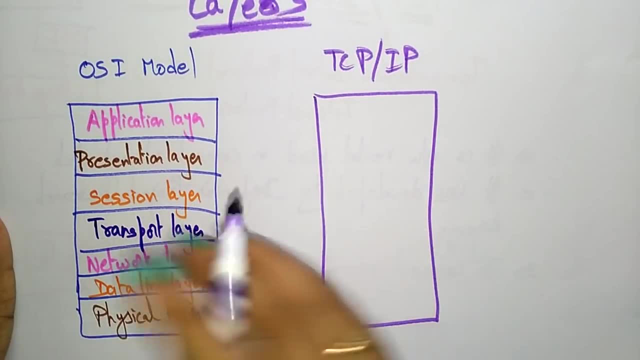 layer. that is the TCP IP model. so in TCP IP model, what are the layers that are present in TCP IP? so here you are having total seven layers, but here in TCP IP you are having only four layers: application layer, transport layer, network layer, and this detailing all. layers. so this is application layer. next, transport layer. so in the place of network layer we call it as a internetwork layer into network layer. so in OSI reference model we use the network layer, that name we use network. in TCP IP we use the name internetwork. 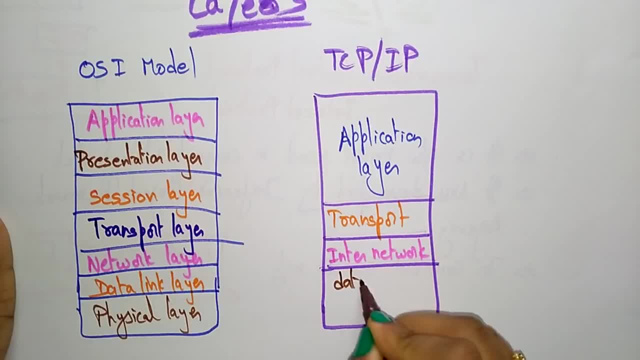 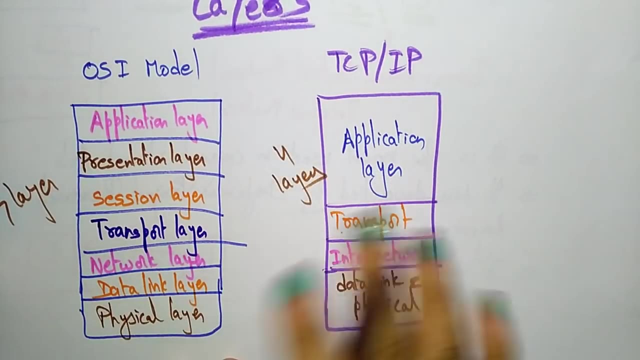 and then layer is the data link and physical layer. both are present in only one layer, occupy the one layer. okay, so here, total seven layers are present in tcp ip are having only four layers. the four layers are present in tcp ip and seven layers in osa reference model. so whatever this, 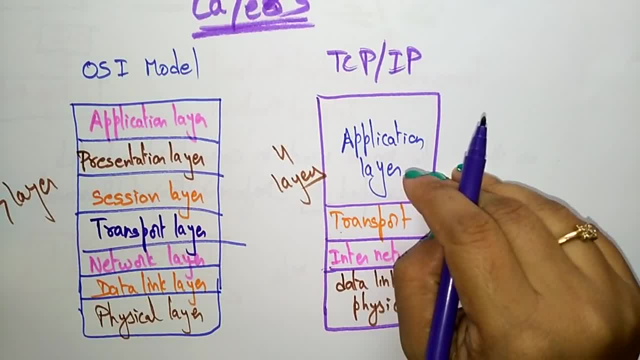 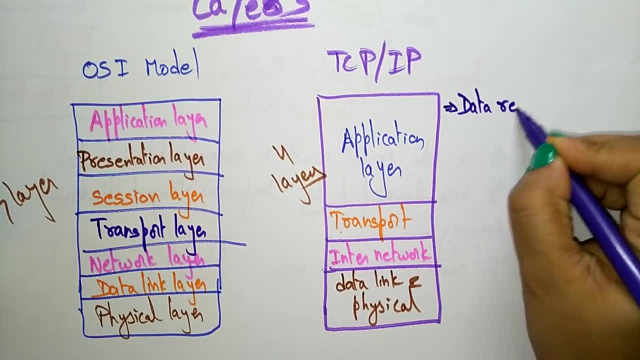 application layer. the application layer in tcp ip is mainly used for data representation. it is used for data representation and uh dialog control and uh application interface, application interface access and application interface and uh. and next, coming to the transport layer. so what is the job of the transport layer? 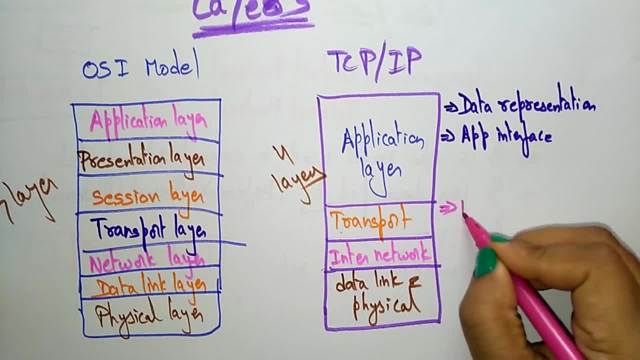 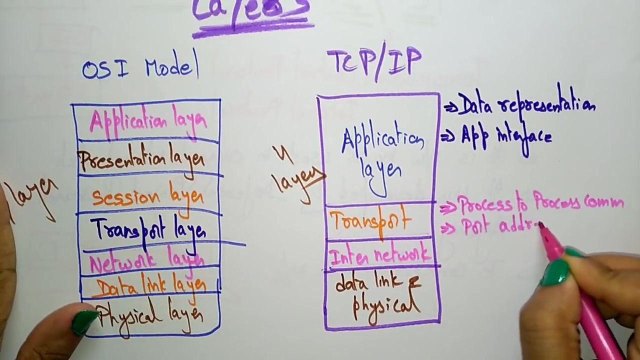 so the transport layer is a process to process communication. so just, it is a process to process communication and here the port address we used for communicating from a system to system, a process to process communication. we use port address, so we need port address to communicate. so just like a transport means if you want to send a